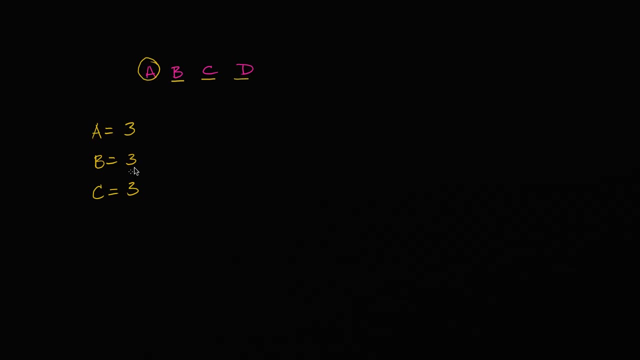 She'll shake the hands of A, B and D, And then, likewise, person D is going to engage in three handshakes, And then likewise, person D is going to engage in three handshakes. So in total you have four people each engaging. 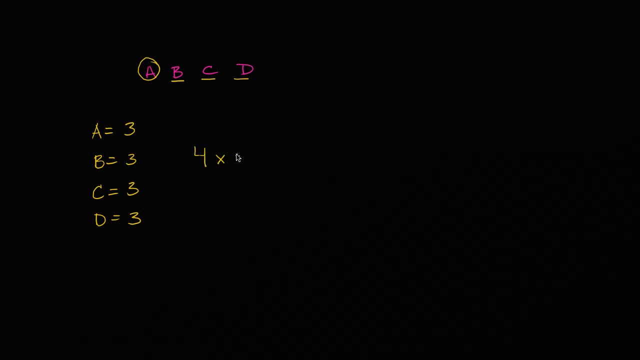 in three handshakes, so you have four people each engaging in three handshakes, so you have 12 handshakes. So my question to you is: do you feel good? do you feel good about this number? Pause the video and try to think about it. 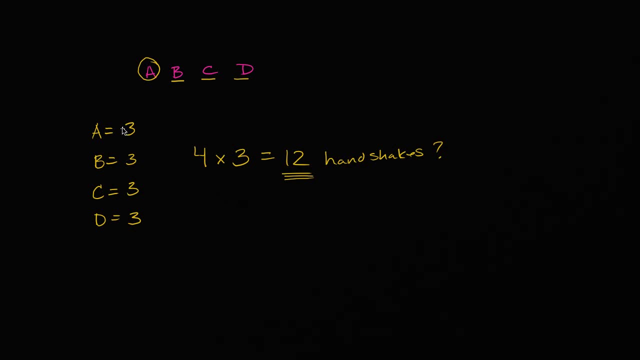 So let's actually draw it out. Let's actually draw all of the handshakes. I kind of went through this argument fairly fast, but I actually want to visually represent each handshake. that goes on, So let's talk about all of the handshakes. 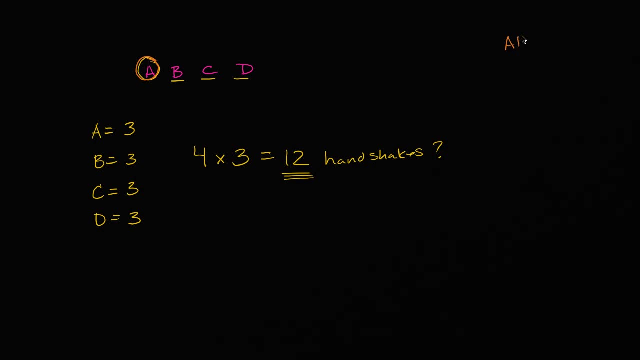 that A engages in. So A is going to shake B's hand, A is going to shake C's hand, A is going to shake D's hand. So it still seems consistent with what we have here, but let's keep going. We're then saying that B is going to shake A's hand. 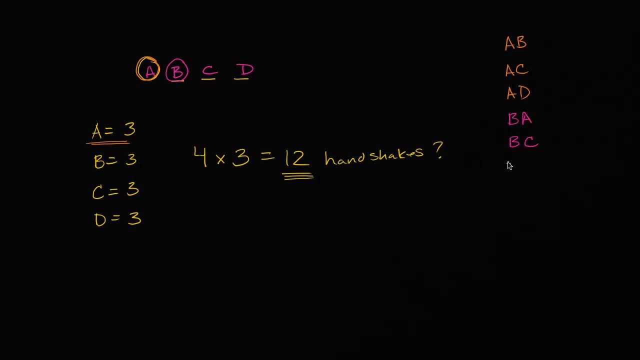 B is going to shake C's hand, and A is going to shake B's hand And B is going to shake D's hand. Now, let's keep going. Then we have C. C is going to shake A, C is going to shake B. 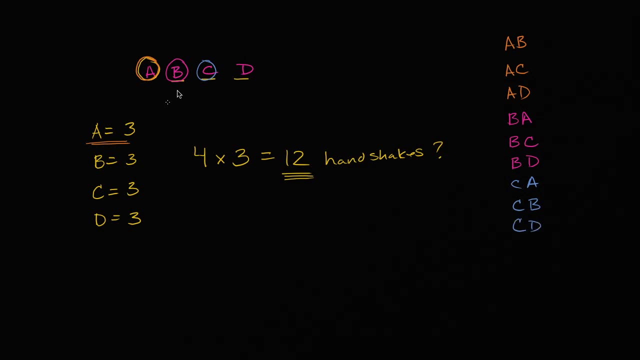 C is going to shake D, And then we have: D is going to shake A's hand, D is going to shake B's hand and D is going to shake C's hand. And you're probably saying: well, Sal, you just listed exactly 12 things. 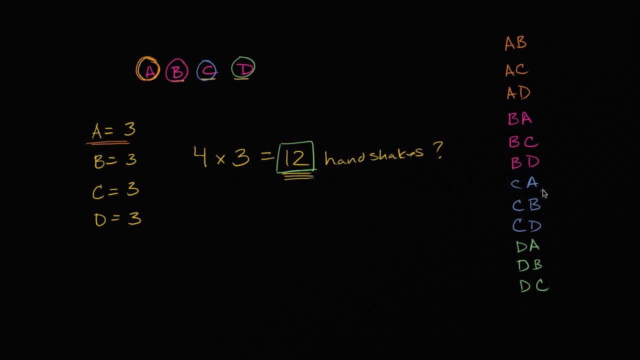 But there's something interesting here: We are double counting And I encourage you to pause the video and think about where are we double counting? So I'm assuming you've had another go at it. But the realization- remember we're saying that each person shakes. 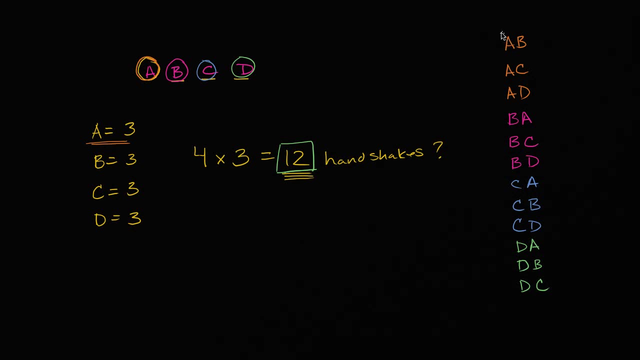 each other guest's hand exactly once. So this is A and B shaking their hands, but this is also A and B shaking their hands, So we have double counted this. It's no different if B is shaking A's hand than A is shaking B's hand. 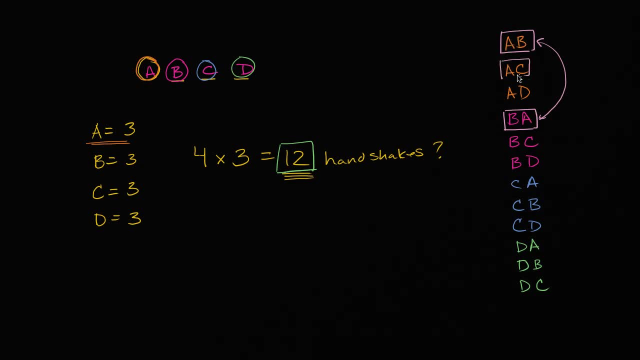 This is exactly one handshake. Likewise A shaking C and C shaking A. this is the same. I guess you could say this is we're either saying that these are two handshakes, even though we're saying that people should only shake their hands once.